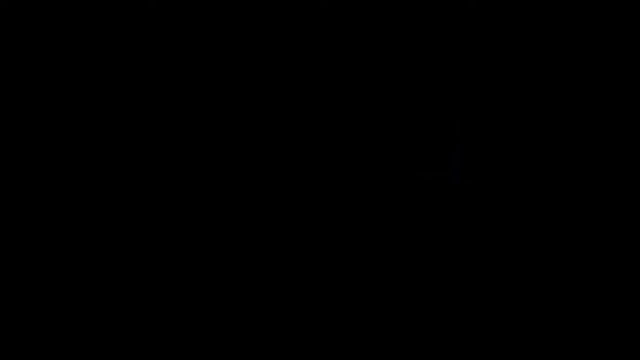 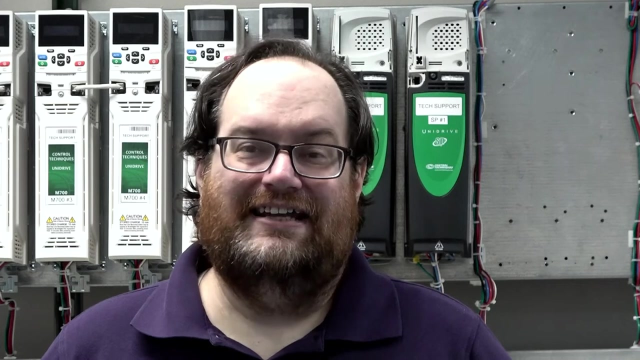 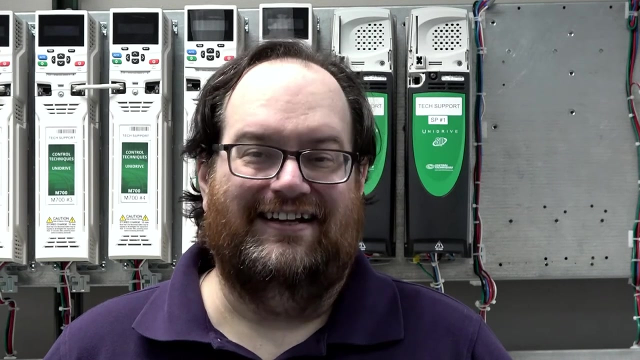 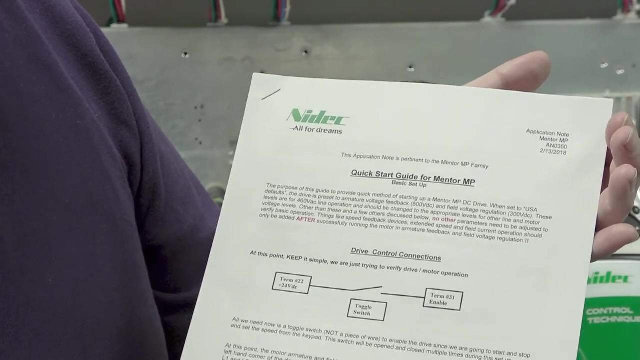 Hi, I'm Shawn Harvey, DC Drive Specialist here at Control Techniques. In today's video I'm going to go over a quick start-up of the Mentor MP DC Drive. So if you're ready, let's get started. In today's video I'm going to be following this guide: the AN0350.. It is. 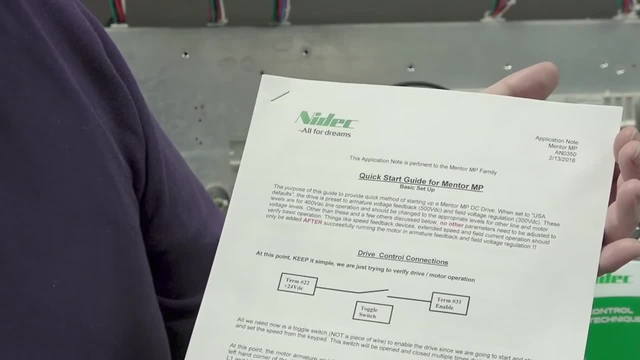 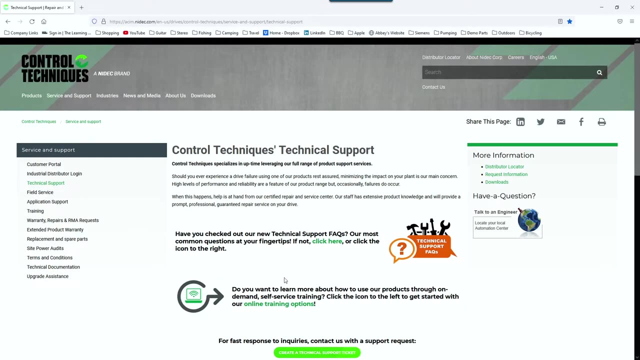 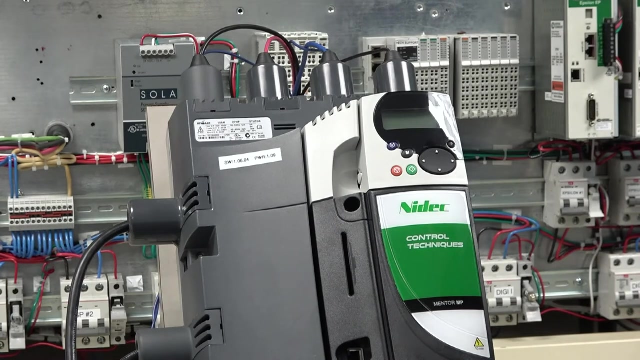 the quick start guide for the Mentor MP. It is downloadable from our website at wwwctdrivescom. before. Before we get started, it's important that you understand we've already followed the instructions in Chapter 4 of the Mentor MP Short Form Guide for Electrical Connections. This guide: 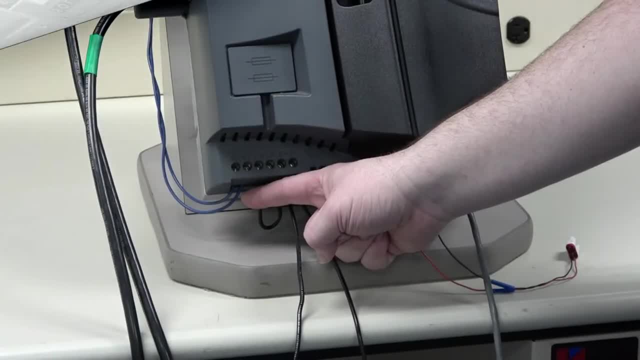 ships with every Mentor MP DC Drive. It is important to note that the terminals E1 and E2 are connected with a DC Drive. They should not be connected in a short form Before We get started. it is important that you understand that the terminals E1 and E2 are connected with a DC Drive. 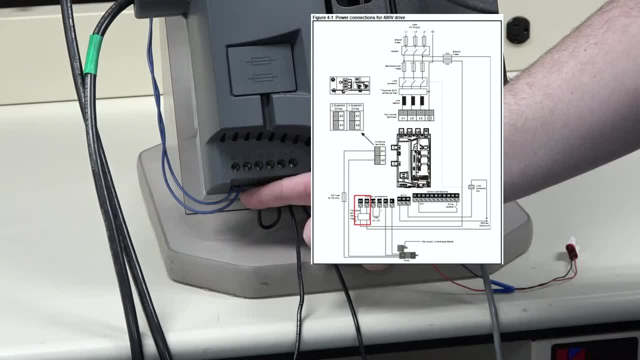 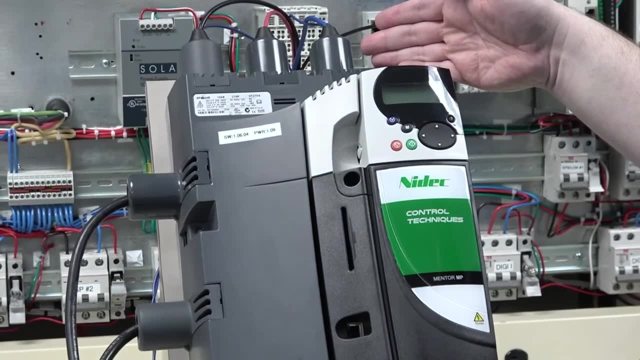 It is important to note that the terminals E1 and E2 are connected with a DC Drive. It is important to are what actually power the Mentor MP DC drive. The terminals L1, L2, and L3 only power the armature. If you have only connected through these three terminals, 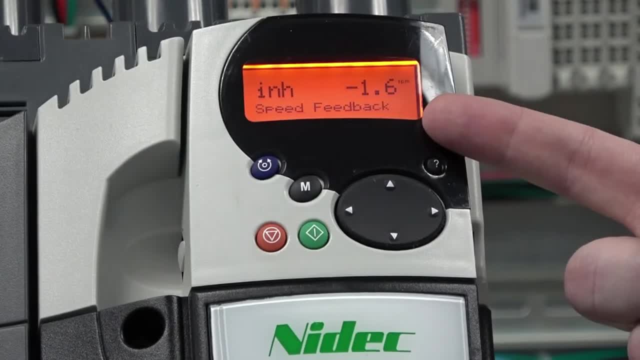 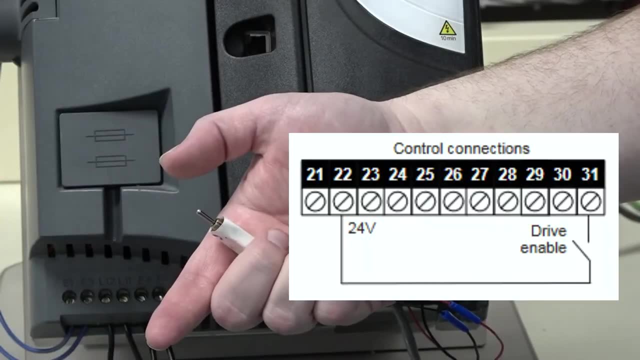 the drive will not power up. I've applied power to the drive and this is what the keypad will look like when it first powers up. You will need an enable switch for the enable circuit, as we will open and close the circuit several times. 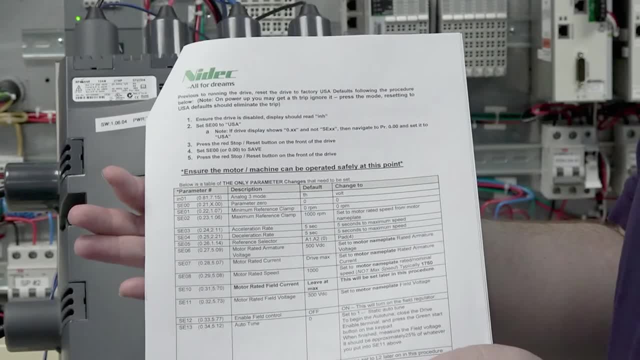 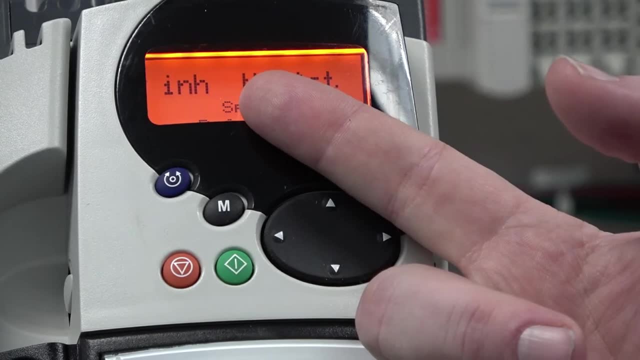 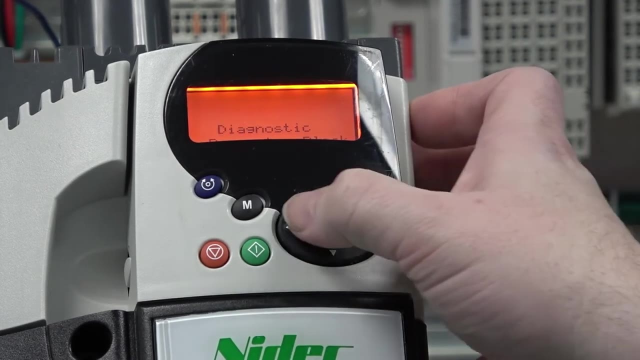 during this procedure. We are starting on page 2.. We will follow each of these steps. Ensure the drive is disabled. The display should read INH. To navigate on the keypad, the left and right arrow keys move you through the different menus. The 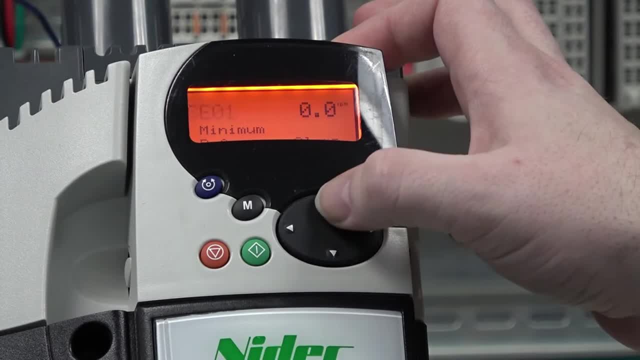 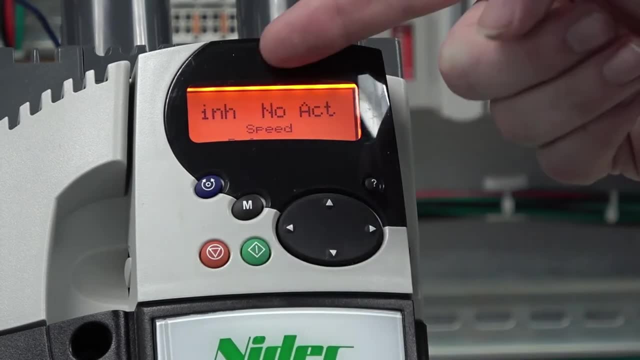 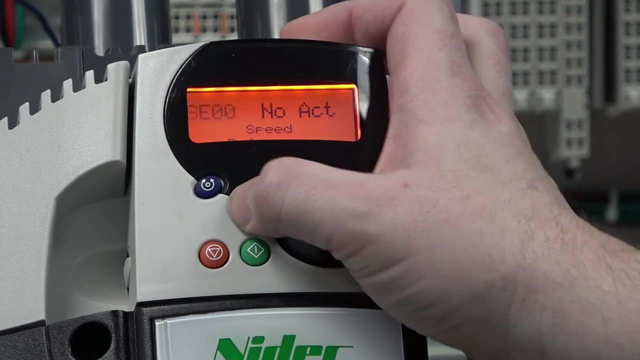 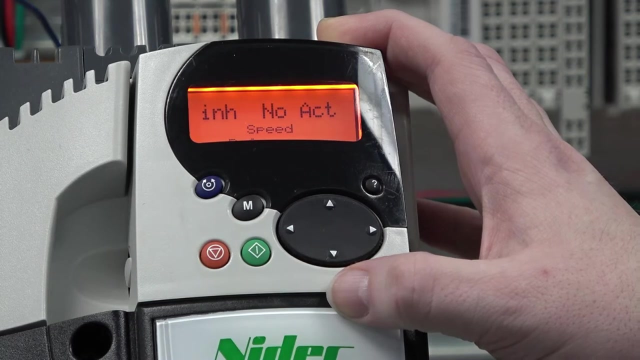 up and down arrow keys move you through the parameters inside the menu you're on. The M button will cycle through the status screen, the parameter navigation and the parameter editing. The first time the drive is powered up from the factory it will be in the sub-block menu. 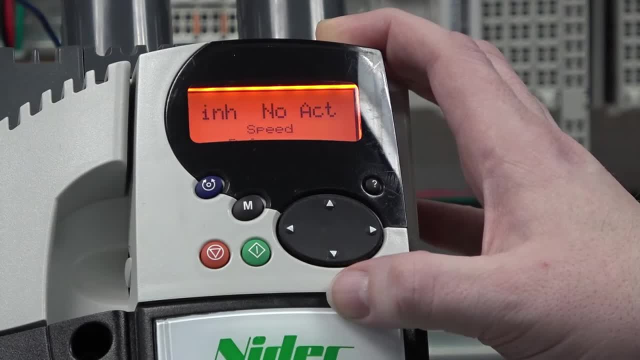 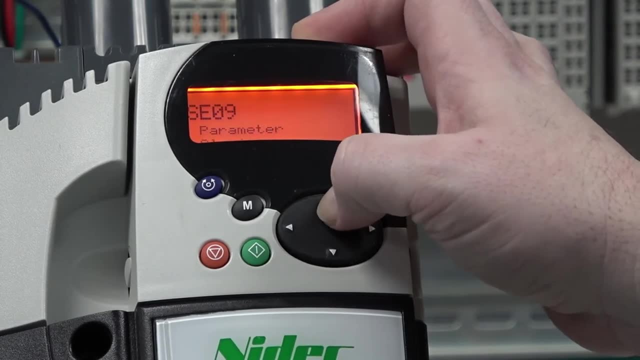 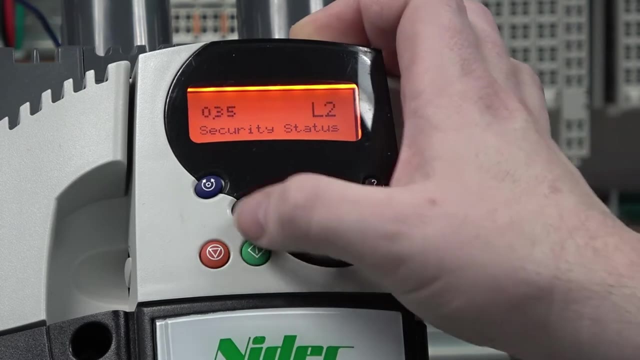 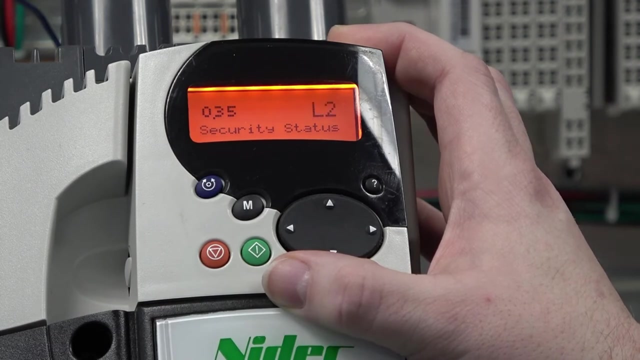 We advise changing the drive to the linear menu structure. To do that, navigate to parameter SE14 and change the value from L1 to L2.. Now that we're out of sub-block mode, the commissioning parameters are in menu 0.. 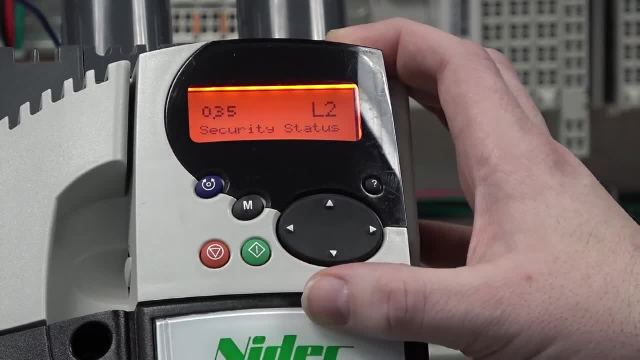 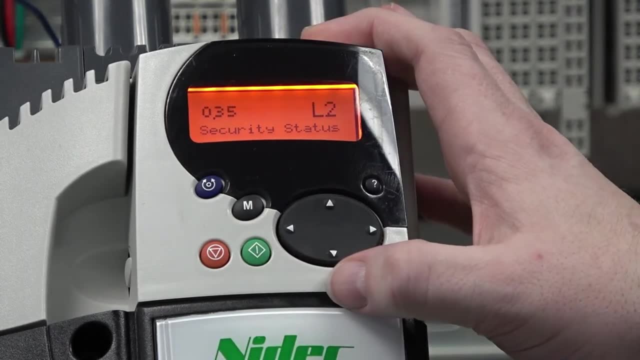 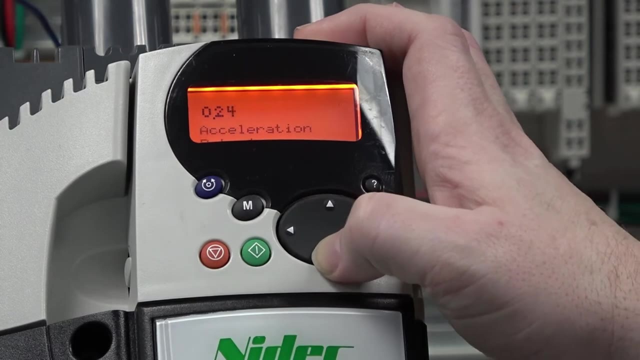 I'm going to use the keypad to navigate to parameter 0.22, which is what we'll start with. First, I'll use the M button to enter parameter navigation. Now I'll use the down arrow key to navigate down to parameter 0.22.. 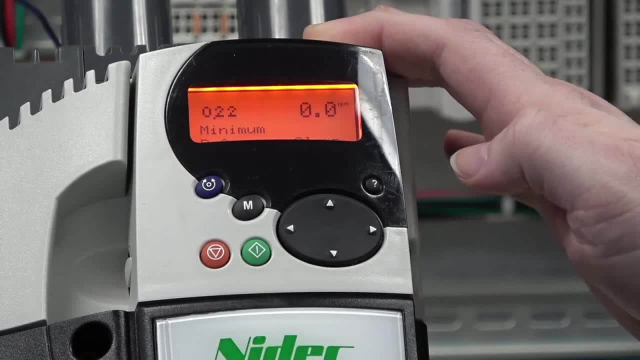 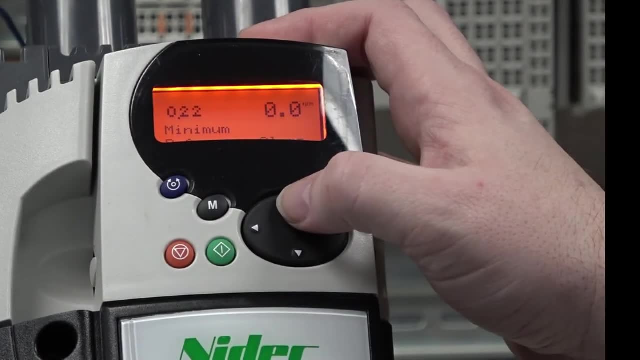 Parameter 0.22 is the minimum reference clamp. Its default value is 0, and for our application that's what we want, So we're good there. Next we'll go to parameter 0.23.. This is the maximum reference clamp. 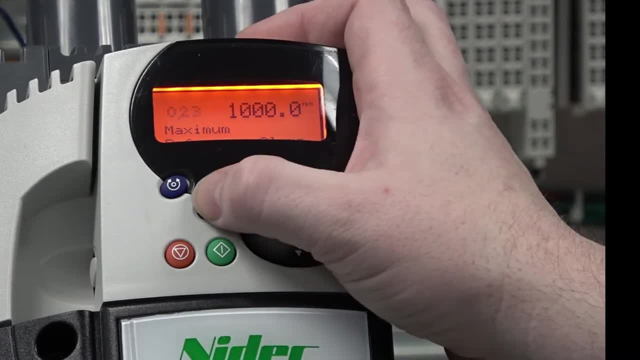 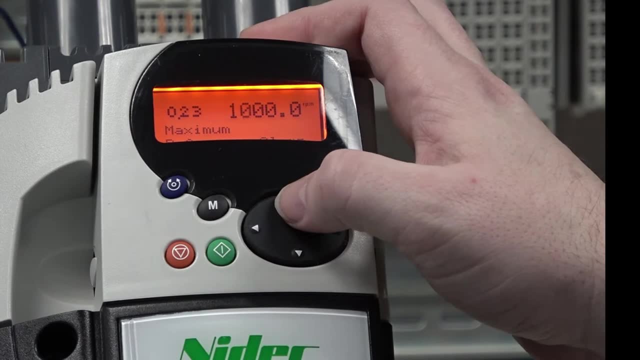 This. I'd like to be 1750.. I hit M to edit the parameter. I use the left arrow key to move the cursor over to the hundreds place. Now, the up and down arrow key edits where my cursor is, And M to go back to parameter navigation. 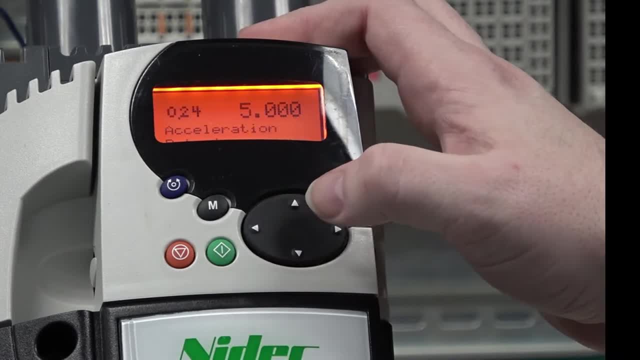 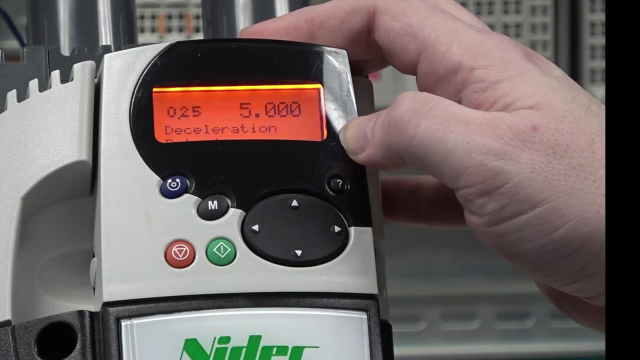 Next up is parameter 0.24.. This is our acceleration rate. I'm happy with the default value of 5 seconds. So on to parameter 0.25.. This is the deacceleration rate. I'm also happy with the default value of 5 seconds. 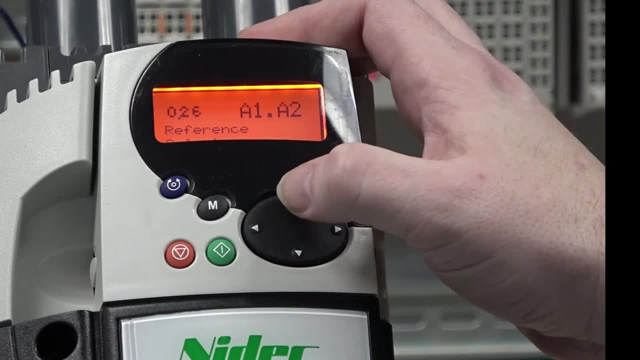 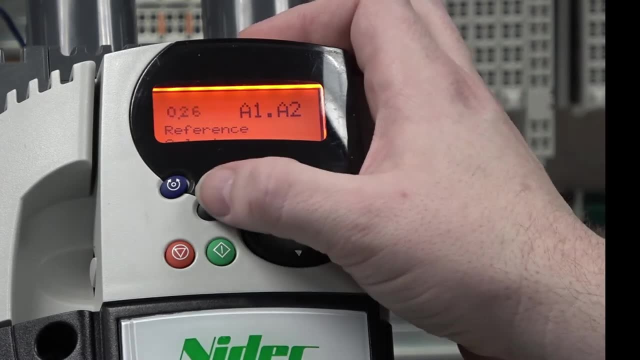 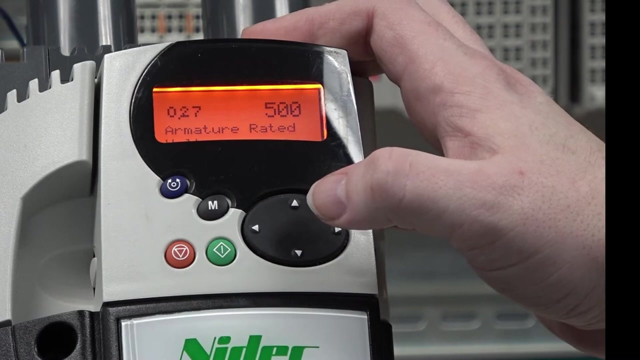 So next parameter 0.26.. This is the reference selector. It tells the drive where it's going to get its speed reference from. We're going to change this to pad so that the keypad controls it. On to parameter 0.27.. 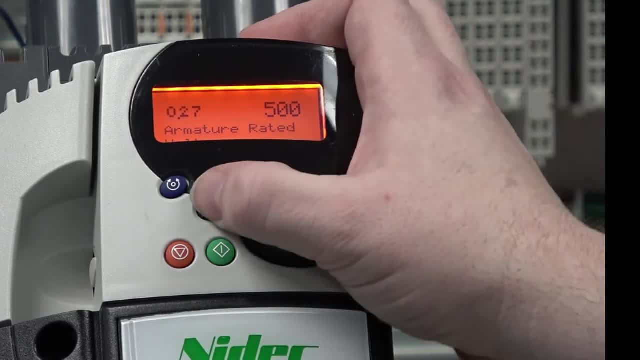 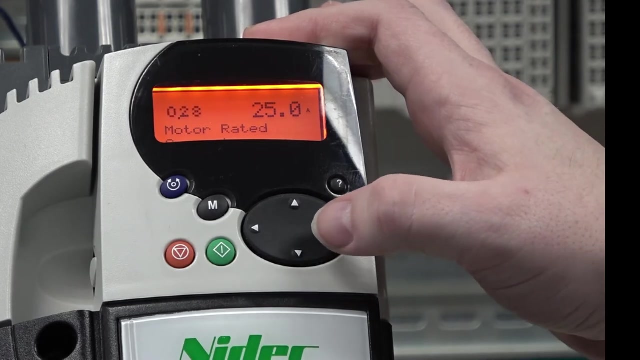 This is the armature rated voltage. Our motor is 180 volts. Parameter 0.28 is the motor rated current. We have a 23 amp armature. We're going to change this to pad. We're going to change this to pad. 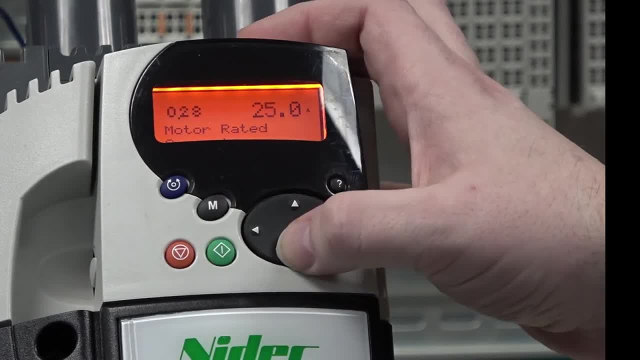 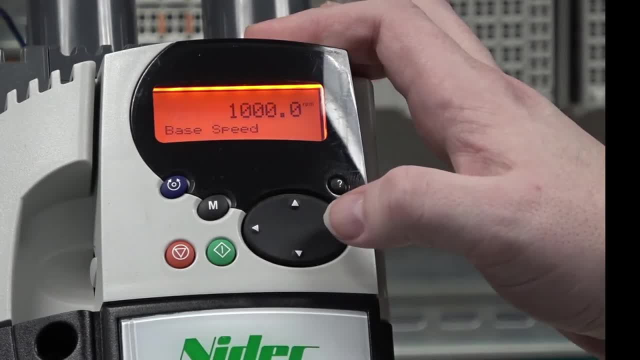 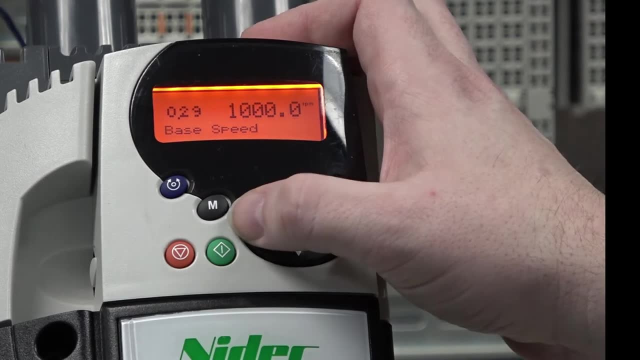 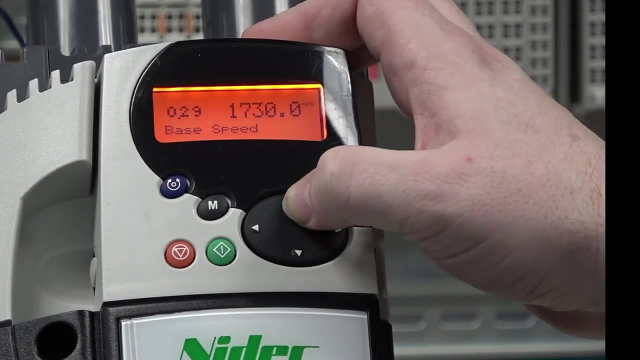 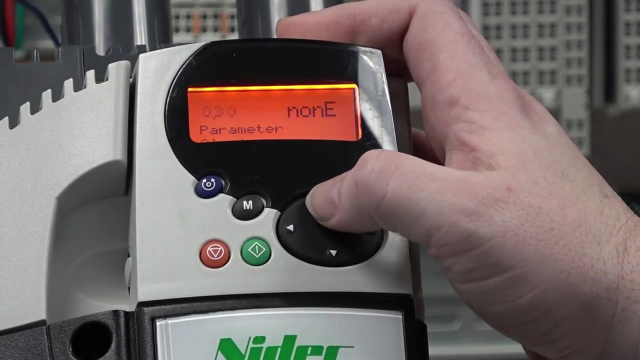 We're going to change this to pad. 0.29 is the motor base speed. This motor is a 1750 RPM motor. Now we're skipping over parameter 0.30.. That's for parameter cloning. 0.31 is the motor rated field current. We'll be setting this on page 3 of this procedure. 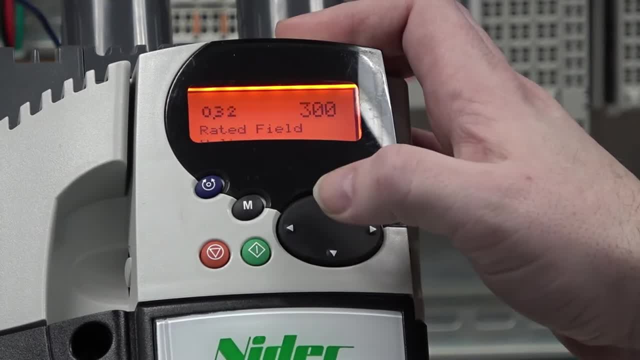 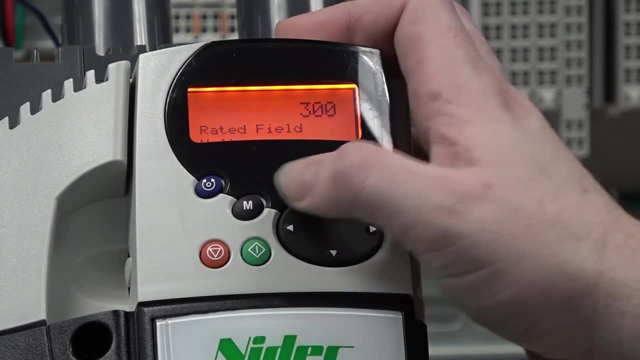 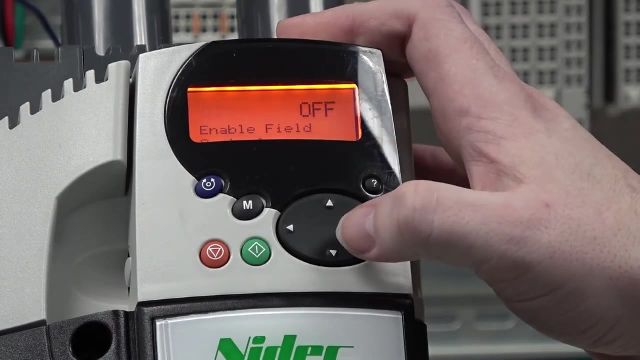 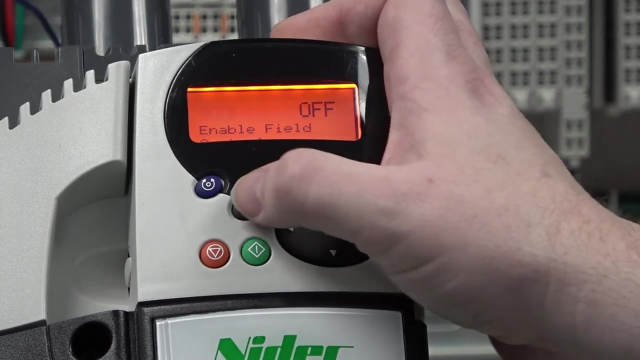 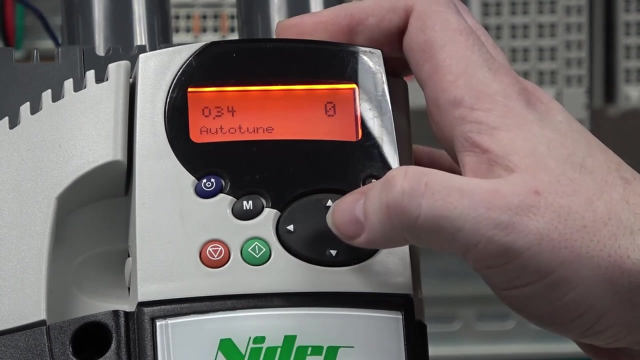 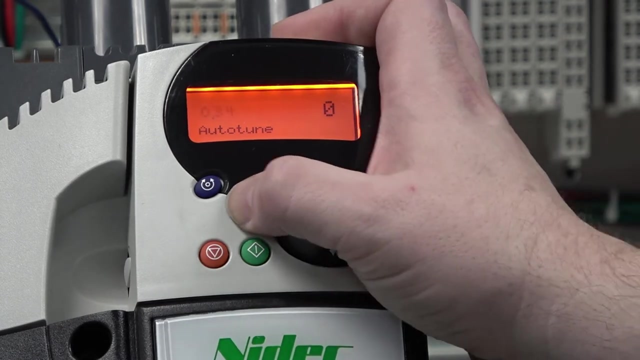 so I'm leaving it at the max value right now. 0.32 is the rated field voltage. We have a 200 volt field. 0.33 is to enable or disable field control. We need to turn our field on now. 0.34 is for the auto tune. You should always perform a static auto tune To do this. 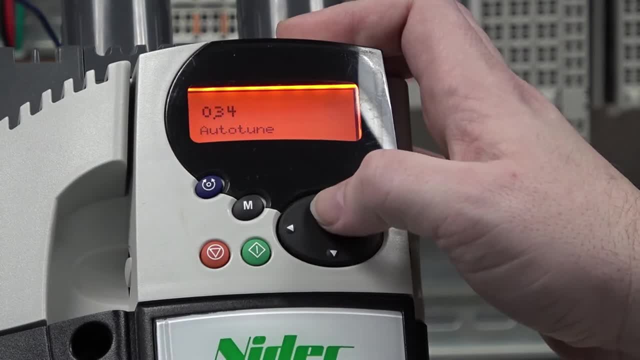 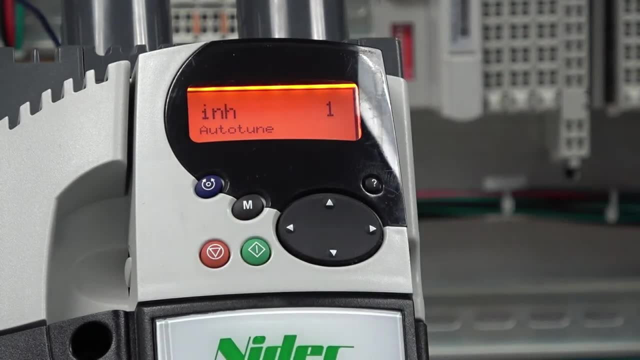 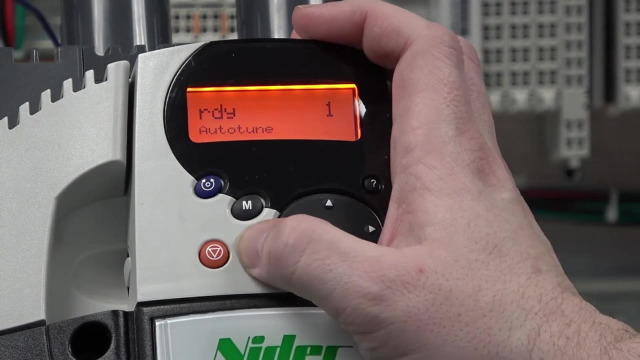 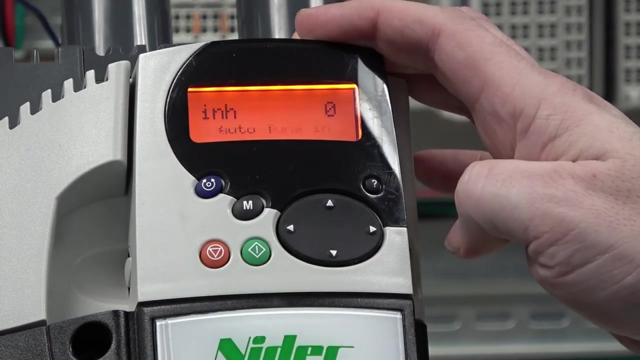 set parameter 0.34 to 1.. Now we're going to enable the drive and we're going to give the driver run command. The auto tune will be complete when that 1 turns back into a 0, like that Now. 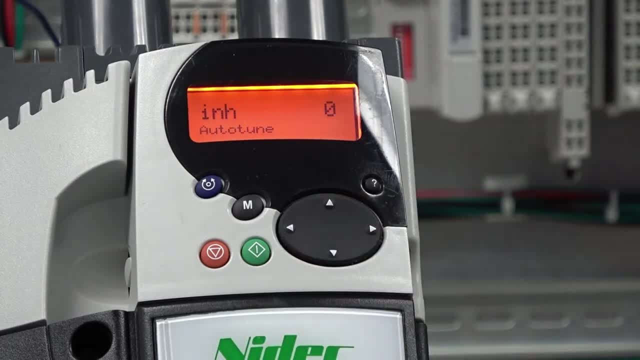 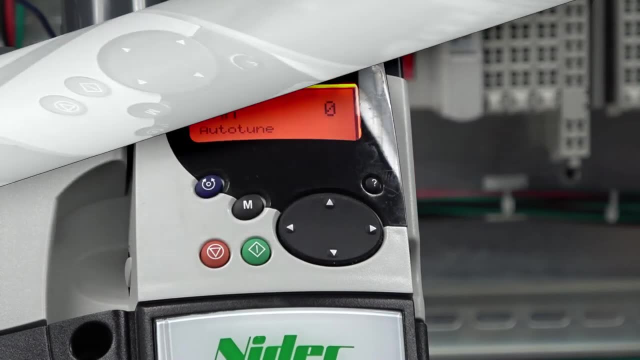 the drive is once again disabled. To get out of this, we need to break the enable circuit and then re-establish it. Now on to page 3.. The first thing we're going to do is run the motor to ensure that the 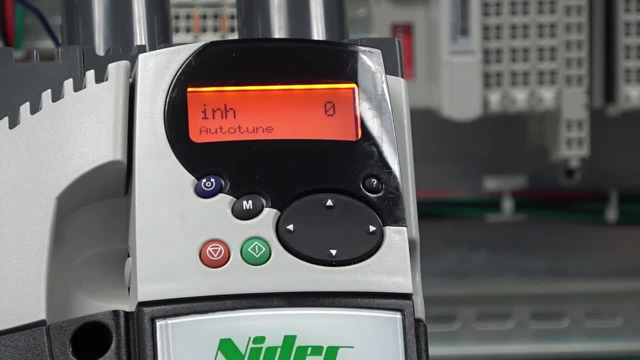 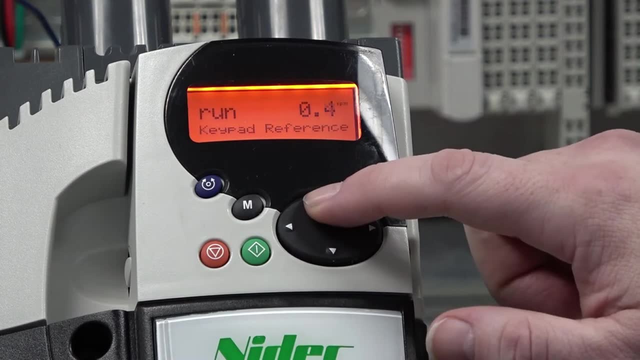 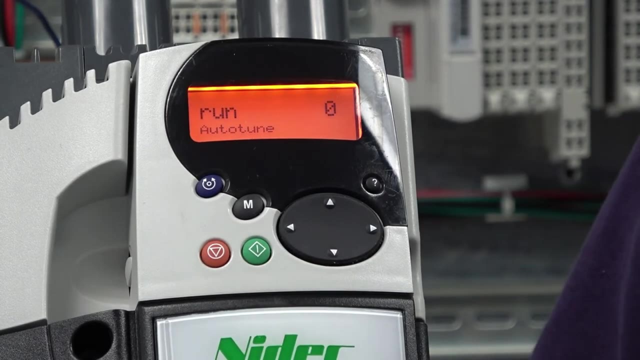 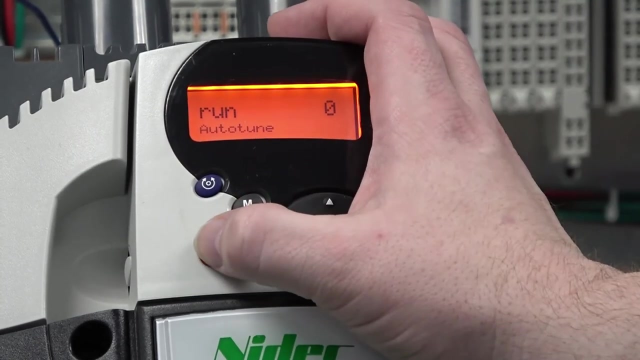 motor rotation is correct for our application. So I enable the drive, I give it a run command, I give it some speed and I observe the motor shaft. We are rotating correctly. Now, if your motor is not running in the correct direction, stop the motor. 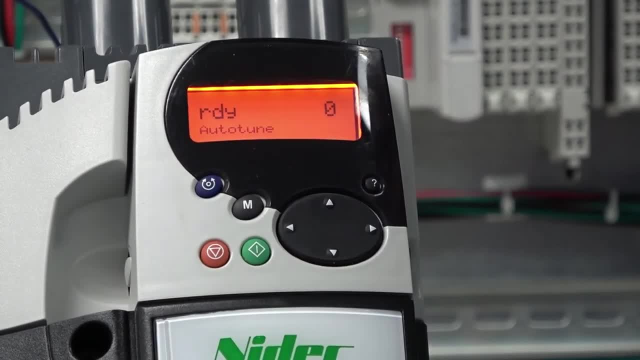 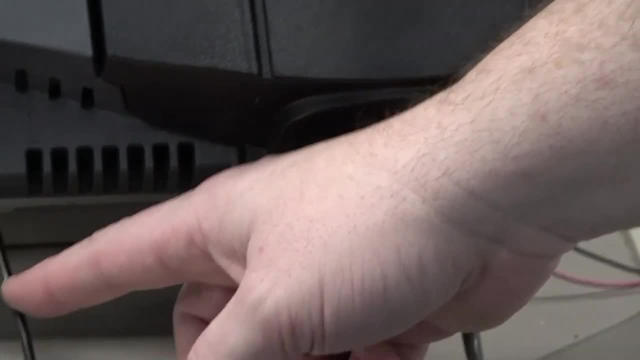 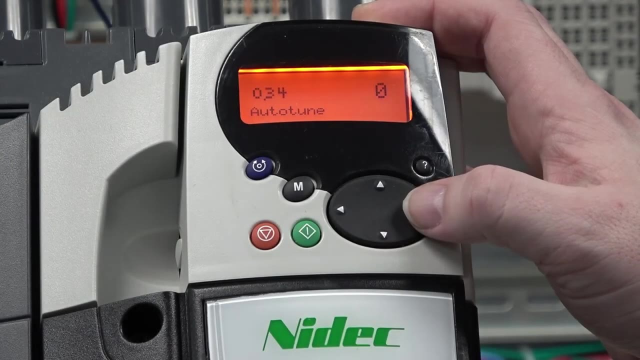 power down the drive and then reverse the two field leads and your motor will then rotate in the other direction. Now we're going to finish setting up the field regulator. To do that, we're going to need to leave menu 0.. 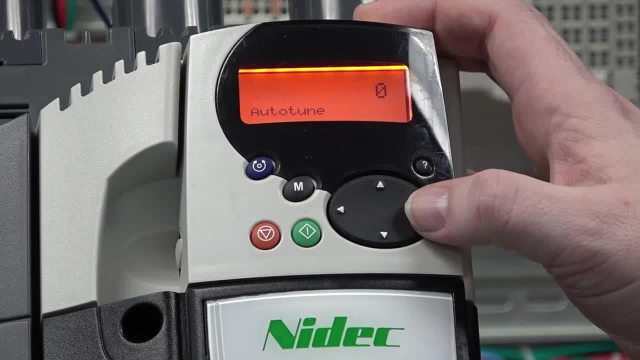 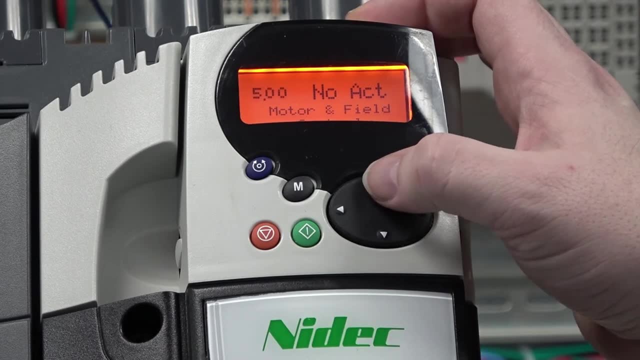 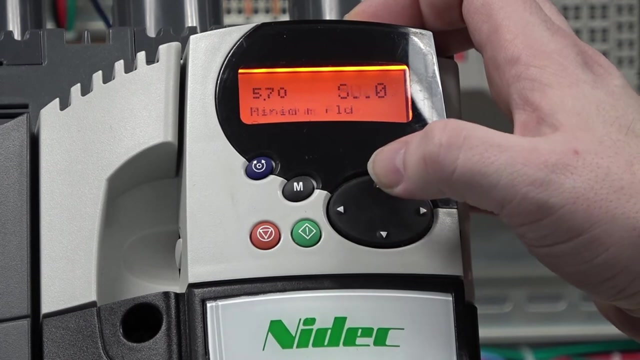 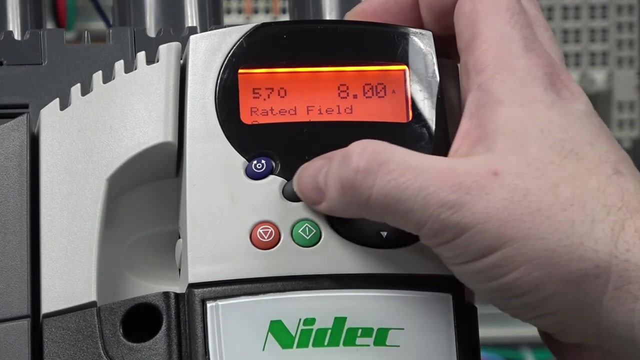 First I'll use the right arrow key to navigate to menu 5.. Now I'll use the up arrow key to navigate to parameter 70 inside menu 5.. This is the rated field. current, Our motor has a 0.1 amp field. 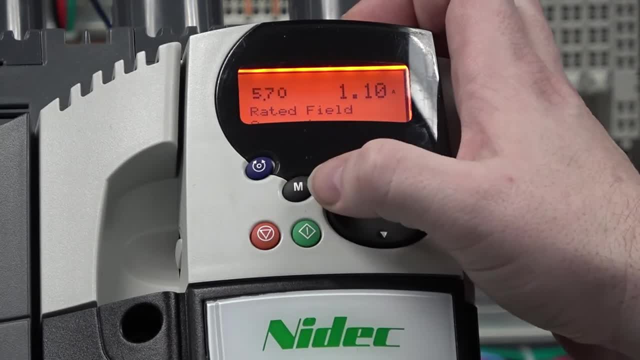 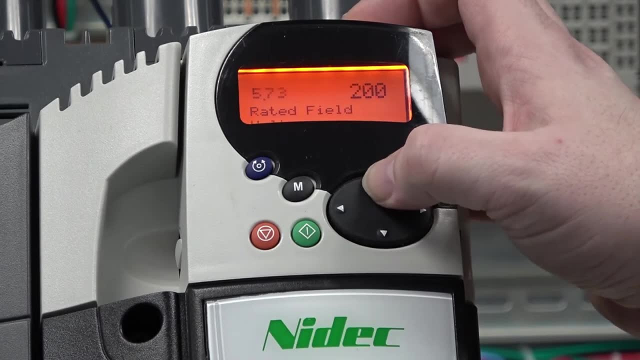 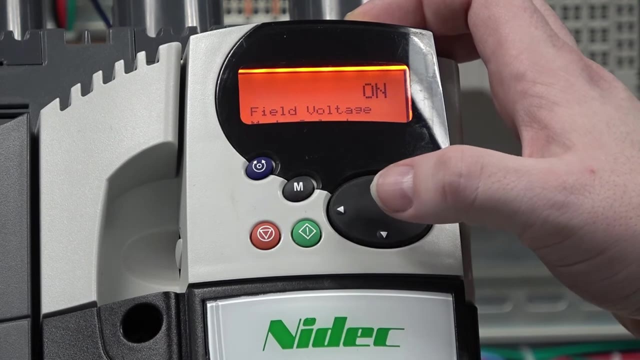 Next navigate to parameter 5.75.. 00000001, 00000002, 000000, Mir vi 5.75. That's the field voltage mode select. It determines whether the field regulator maintains the voltage or the current. We want it to maintain the current, so we want to do that In order to 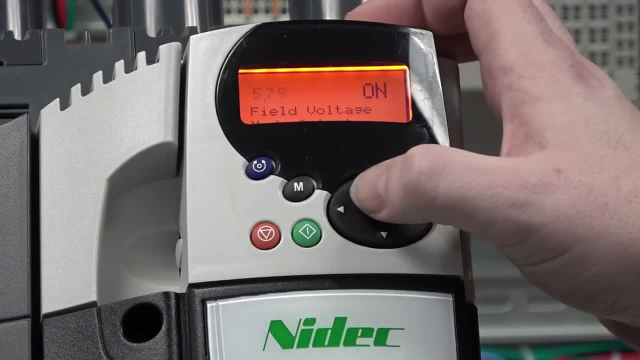 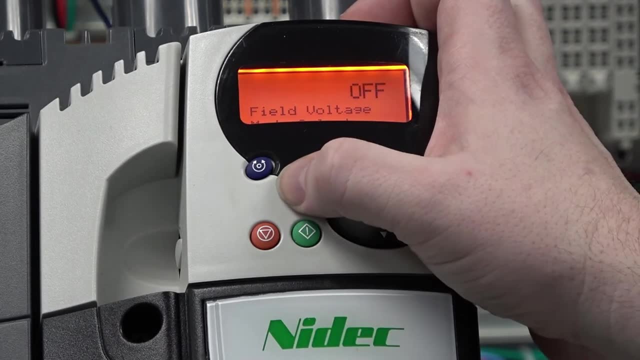 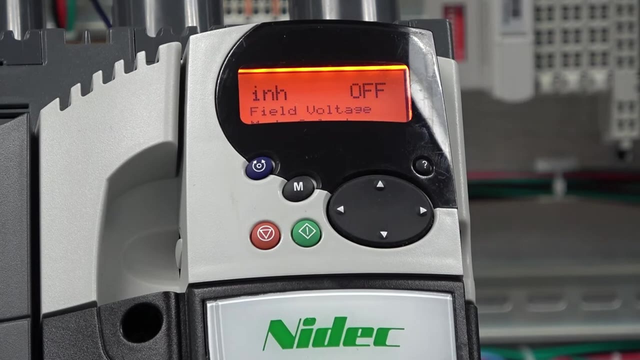 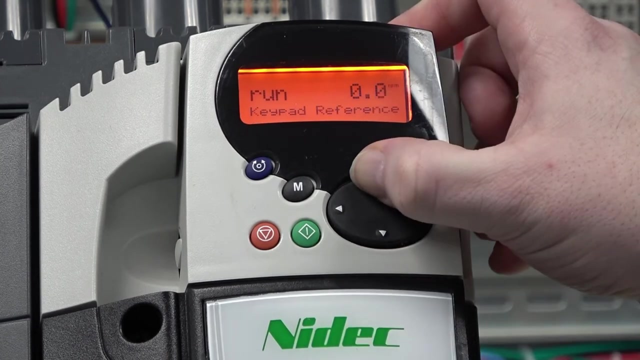 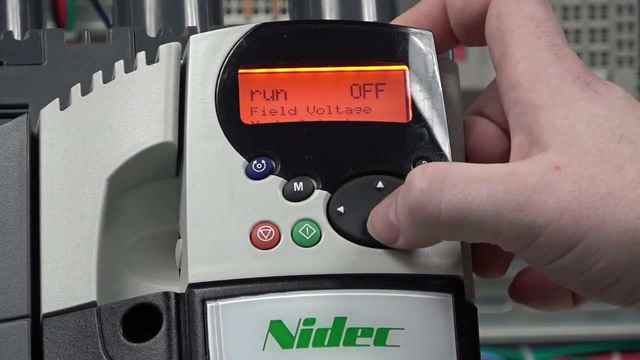 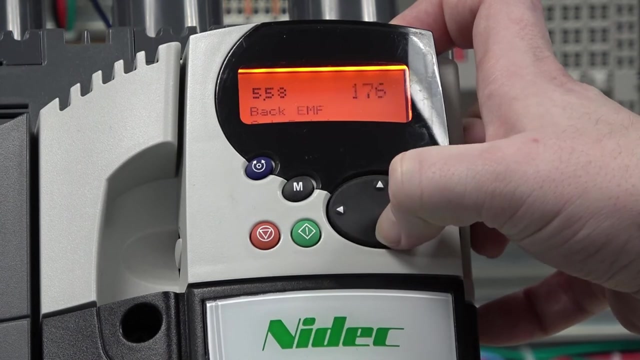 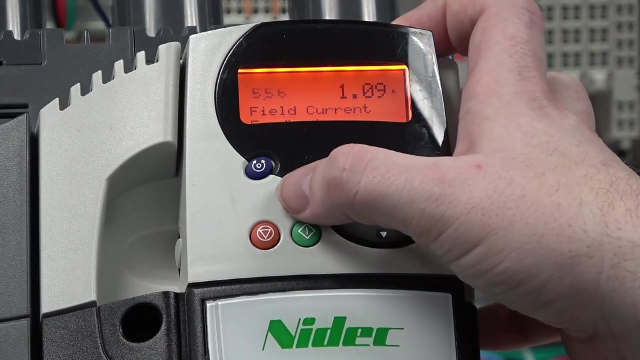 За边iren the current. So we turn it off. So I'm enabling the feel, or I'm enabling the drive, giving it a run command, give it a little bit of speed. and now we're going to look at parameter 5.56.. 1.09 amps- Pretty good. We'll also check the voltage Go to. 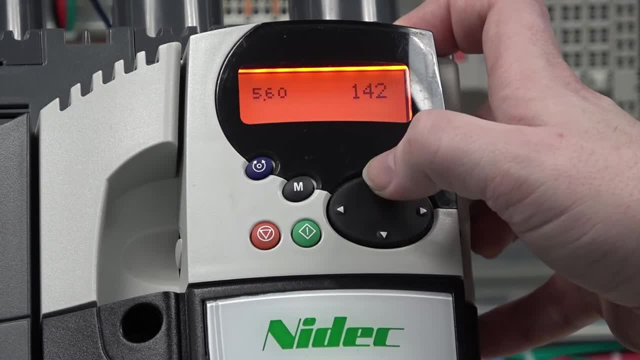 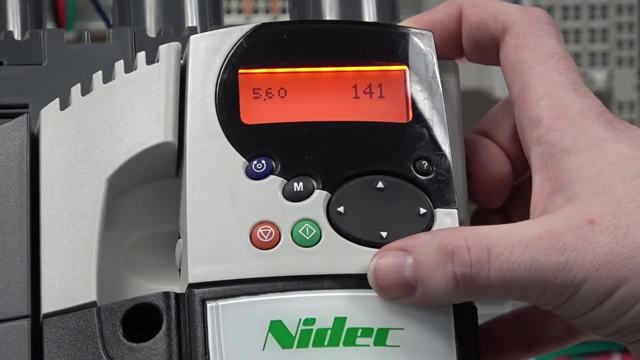 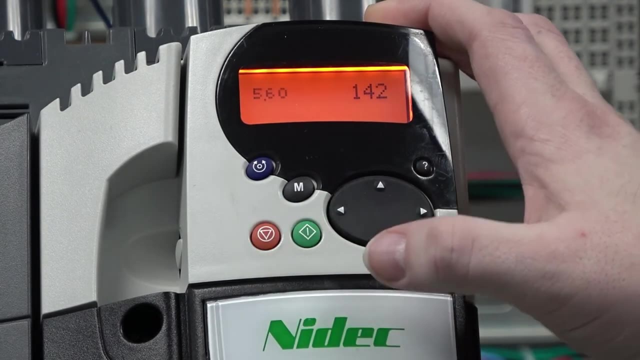 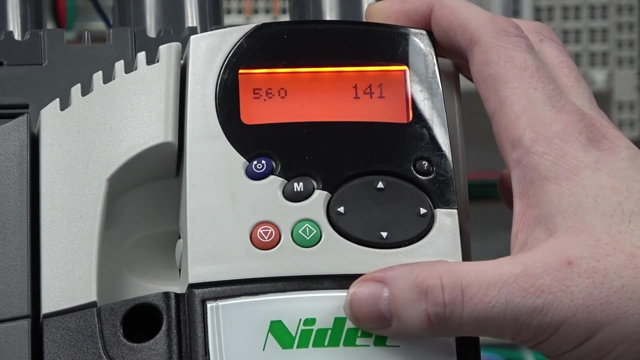 parameter 5.60.. About 140.. 42 volts To be expected when operating in current control mode. Now stop the motor. While we were still in menu 0, all the changes we made saved automatically. Because we're now in menu 5, we have to manually initiate a parameter save To do that. you navigate. 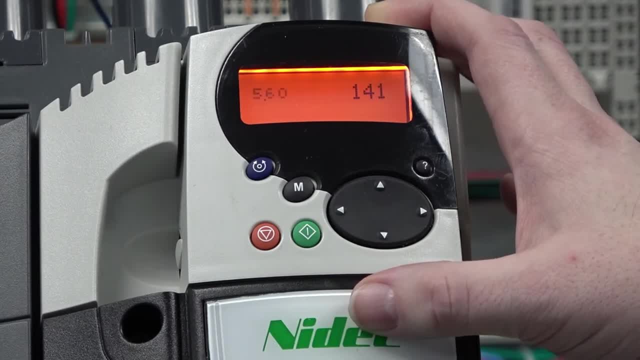 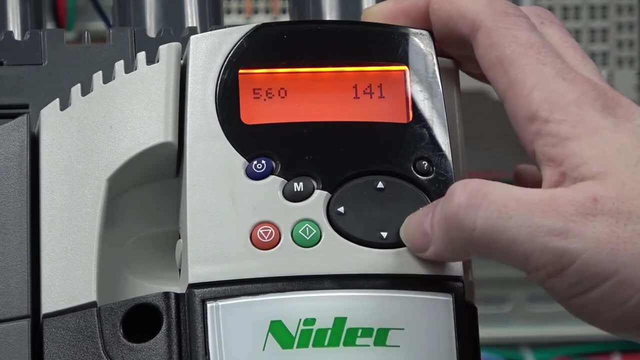 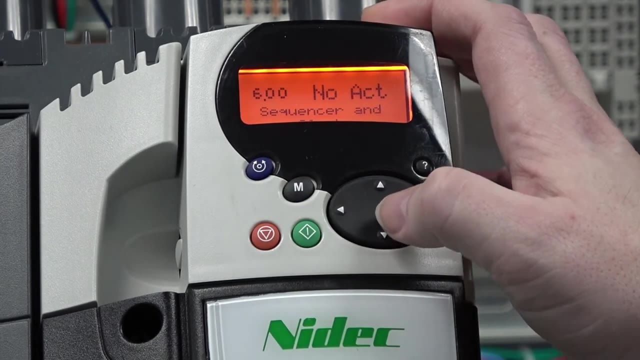 down to parameter 0.0.. However, any parameter 0.0 in any menu has the same effect. So instead of going down 60 parameters, I'm going to hit the right arrow once and be at parameter 6.00.. Now I hit the M button to go into edit mode. I press the up arrow once. 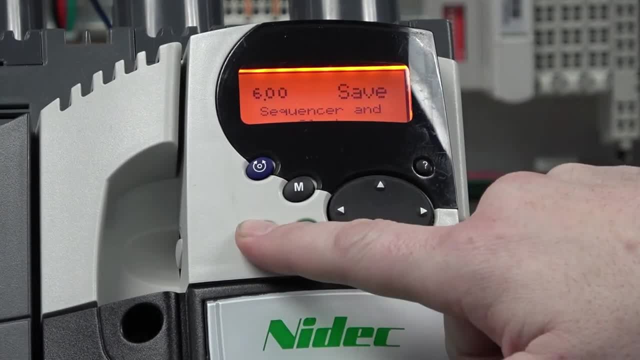 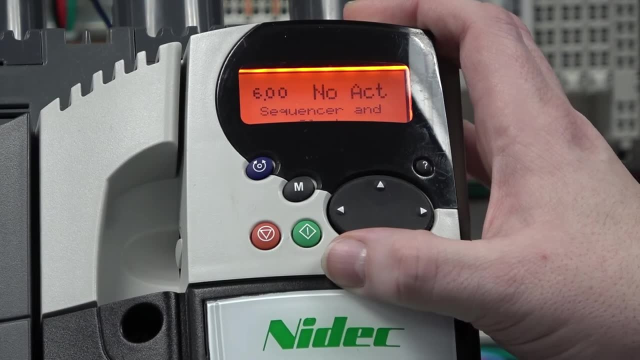 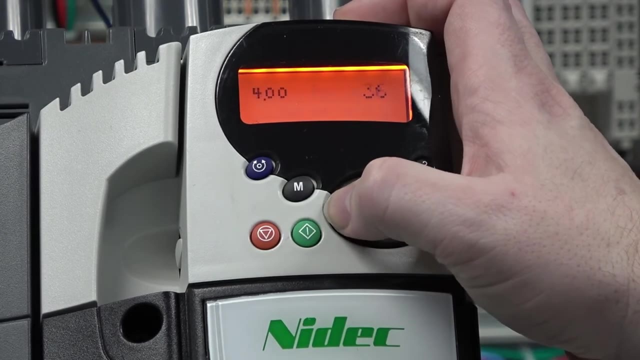 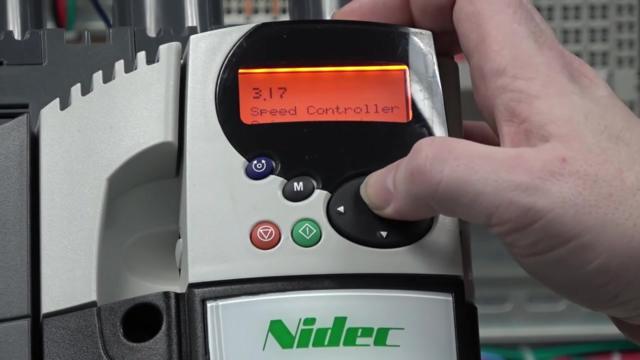 to the option that says save, And I hold in the red stop reset button until the keypad goes back to saying no act. Now we're going to set up speed feedback. Speed feedback can be found at parameter 3.26.. So first we navigate back to menu 3. And then up to parameter 26.. 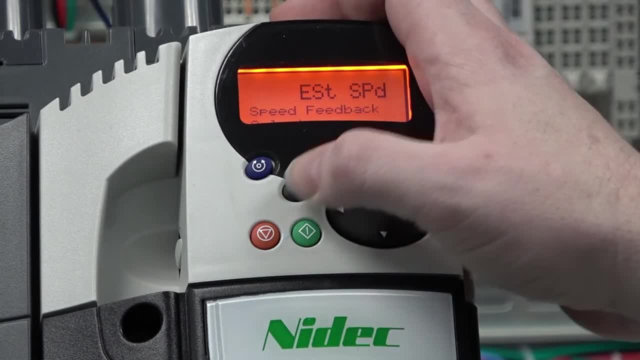 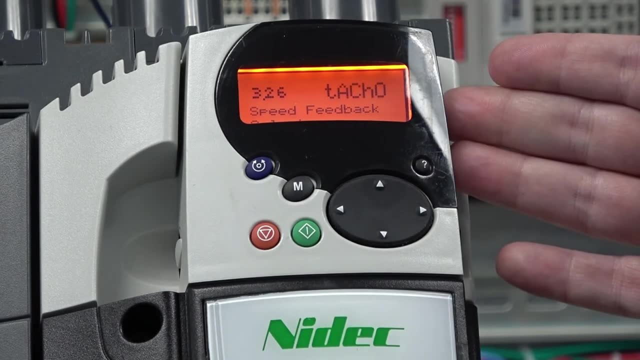 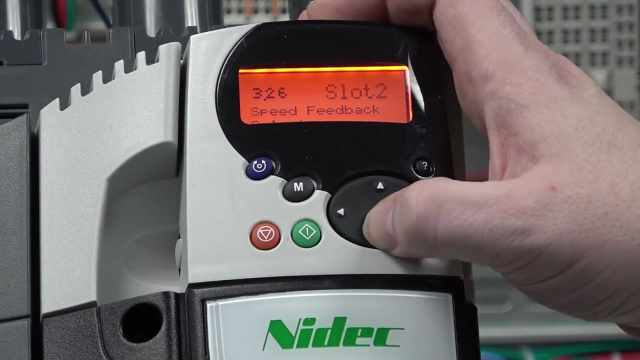 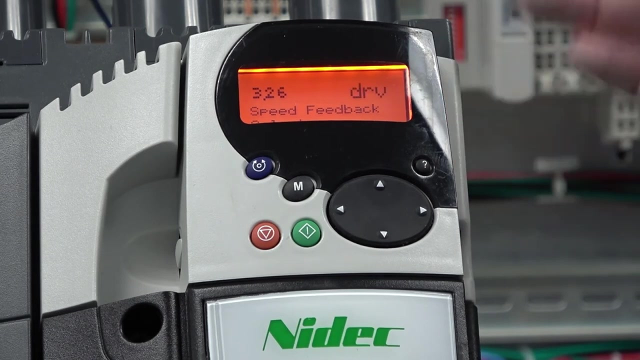 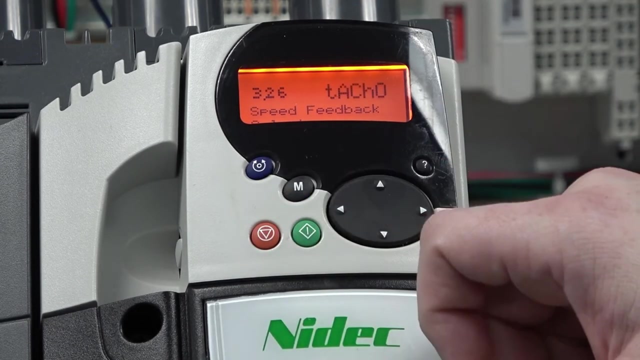 Estimated speed is the default setting. TAC feedback, the instructions for which are found on page 4, is what we're going to use for this example. There's also encoder feedback, which will be found on page 5 of the application. 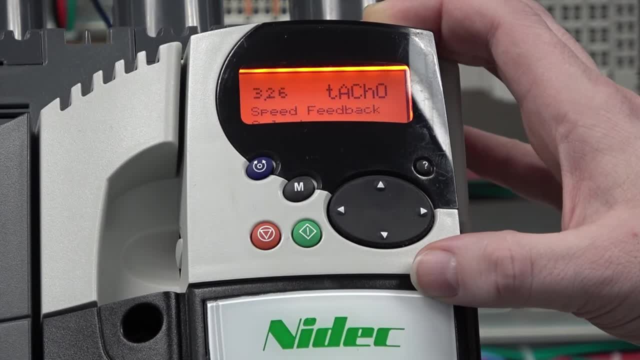 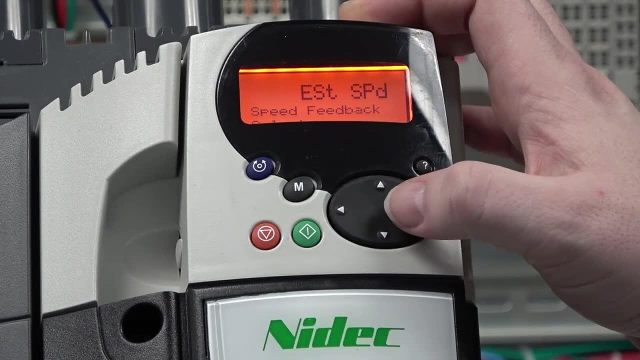 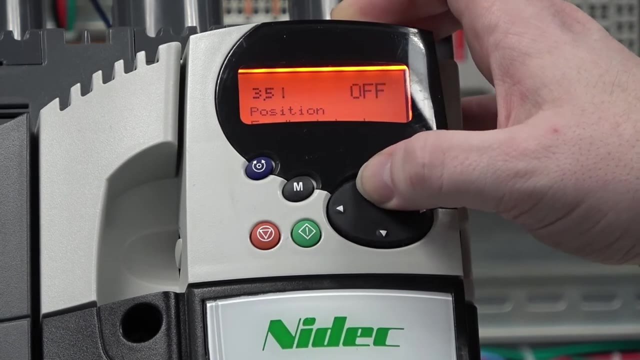 To set up our TACO generator, we actually need to start out in estimated speed mode. Then we're going to navigate to parameters 0.0.. Then we're going to go to parameter 3.51.. This is the voltage per thousand RPM rating of the TAC. 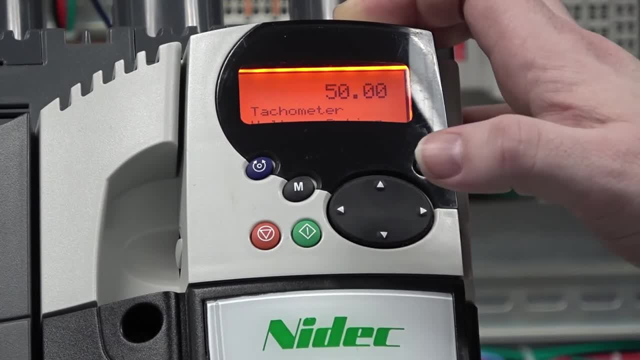 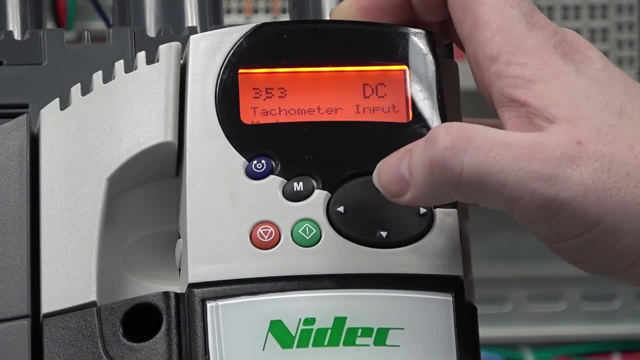 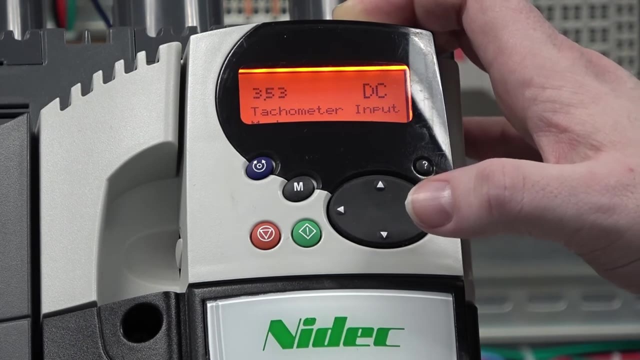 Our TAC produces 50 volts per thousand RPM. That's the default setting. So next we're going to go to parameter 3.53.. This is where you can set what sort of TAC you have. The drive's happy with either an AC or a DC TAC. but do note if you have a regenerative. 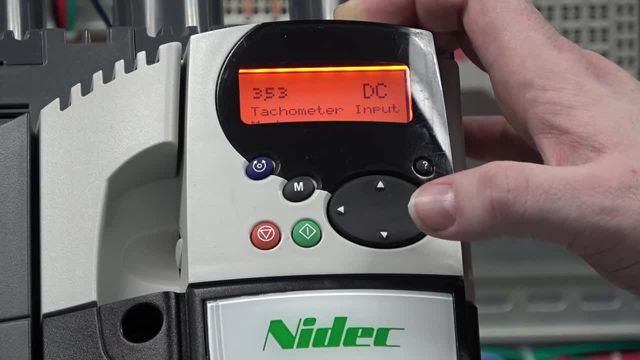 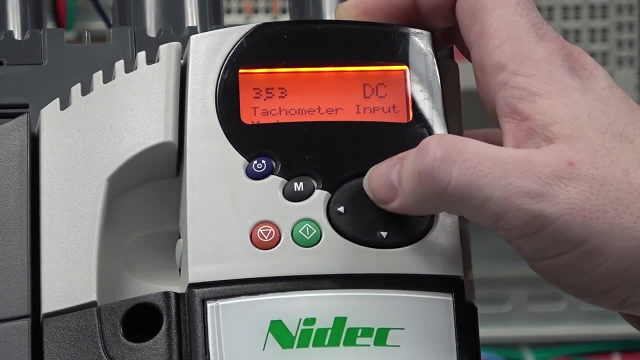 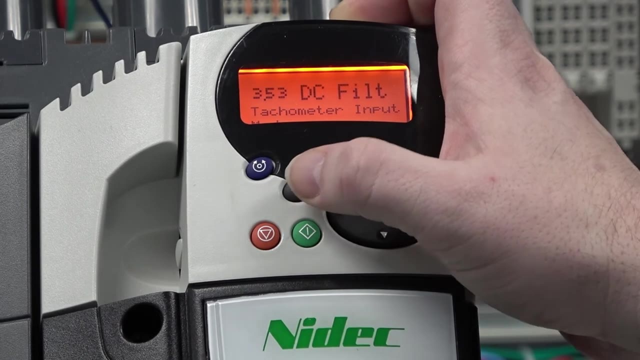 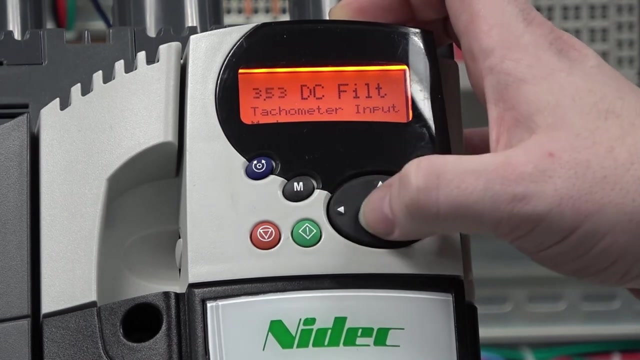 DC drive, as in it will spin the motor in both directions. don't use an AC TAC. It's also useful to use the DC filter setting when you do have a DC TAC. Now we're ready to test, So first I'll navigate to 3.52..